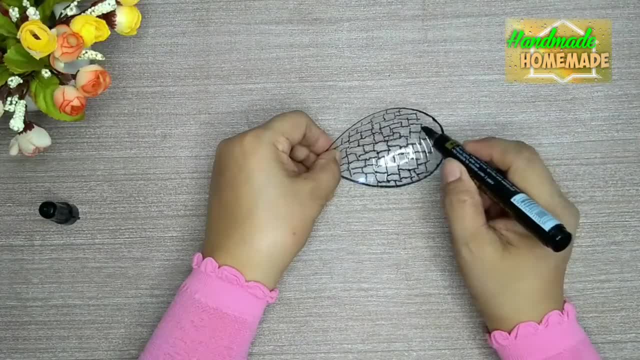 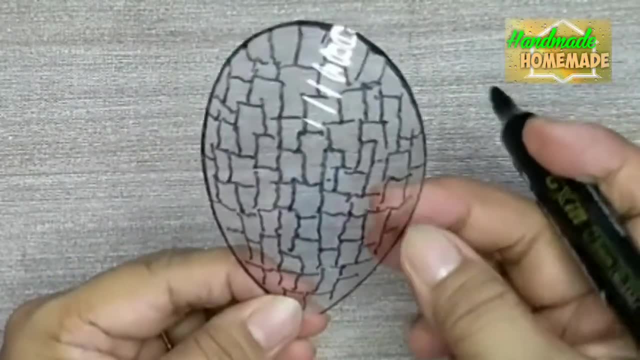 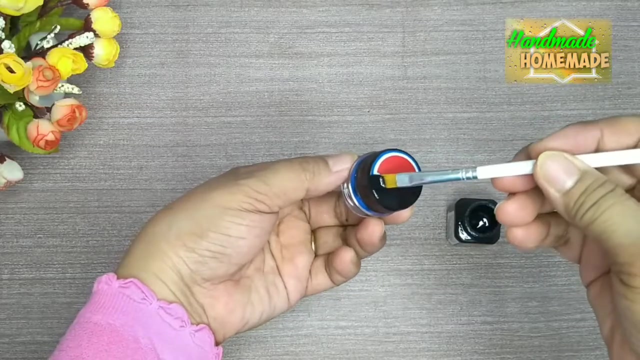 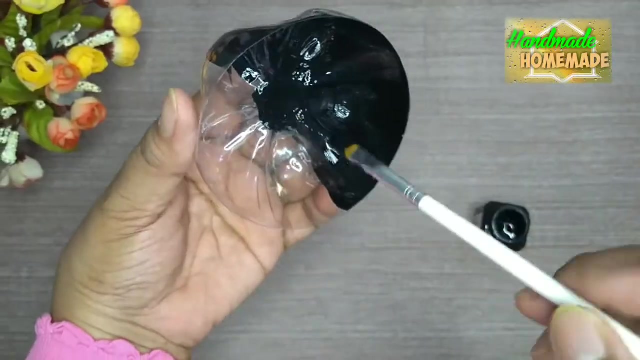 Prophesy like Jeremiah: pray just like Elijah. I'm gonna dance like David. have faith like Abraham. Prophesy like Jeremiah: pray just like Elijah. You're so good, You're so good to me and I can't even even speak. Sometimes, all I can do is cry. 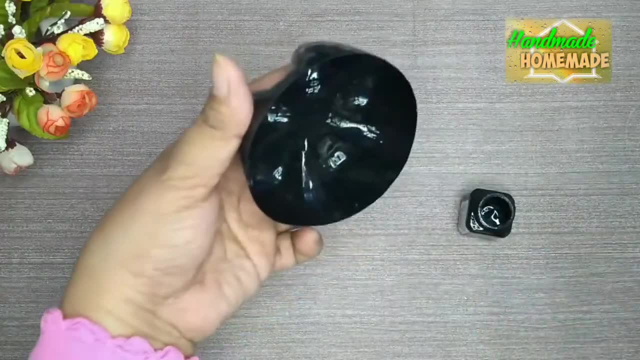 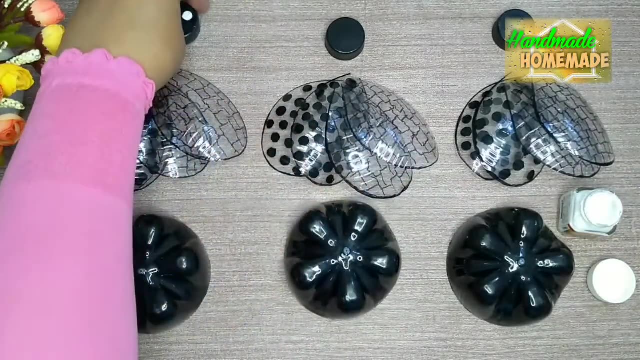 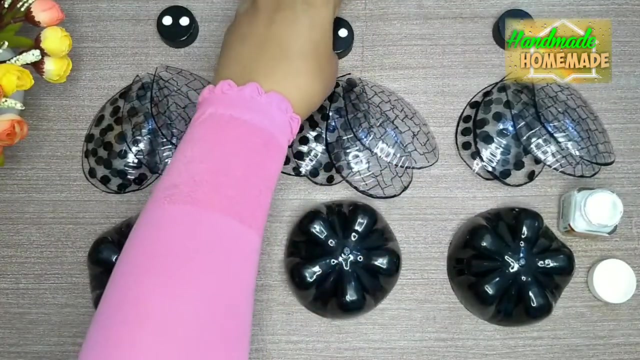 Close my close my eyes, raise my hands, do a dance for you, Praise you, it's true, to the one it belongs to. Thank you, Lord, for all you took from me, for all you've done for me, for how you love me. 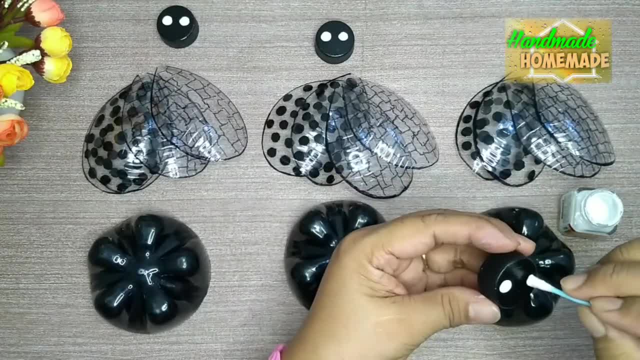 Thank you, Lord, for how you cared for me. you always there for me. Thank you, Lord, for how you cared for me. you always there for me. you said you'd never leave me. Thank you, Lord, for how you cared for me. you said you'd never leave me. 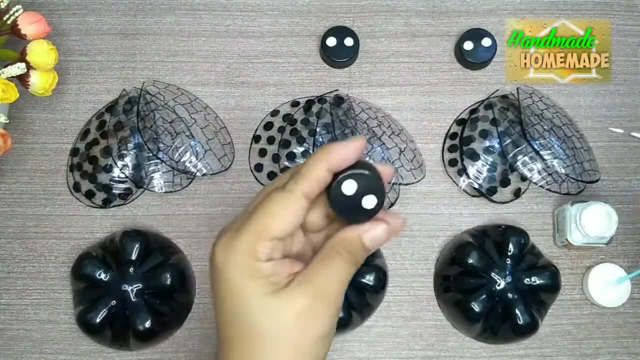 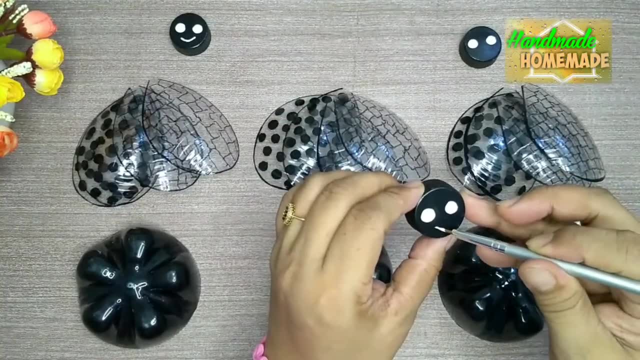 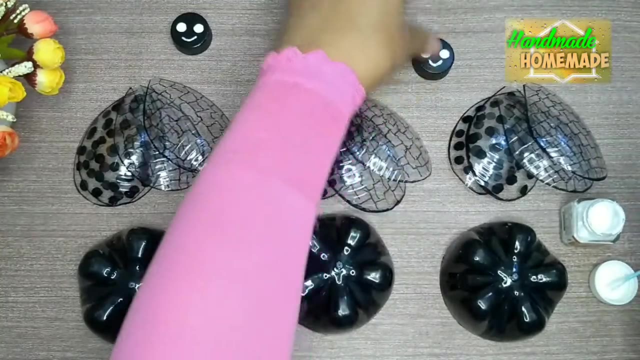 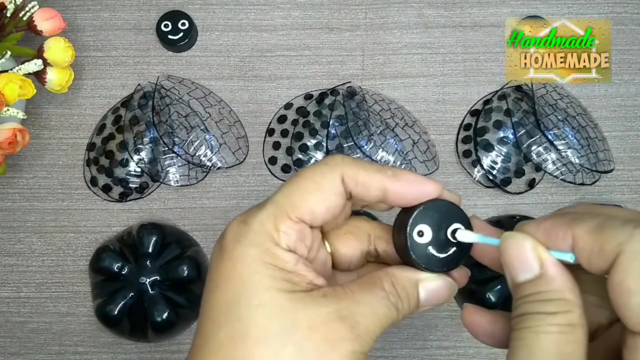 I just wanna never mind, never mind All the things going on in my mind. yeah, Never mind, never mind Right now, just wanna thank you. What do you do? what do you do when you're going through going through? What do you do? what do you do when you're going through going through? 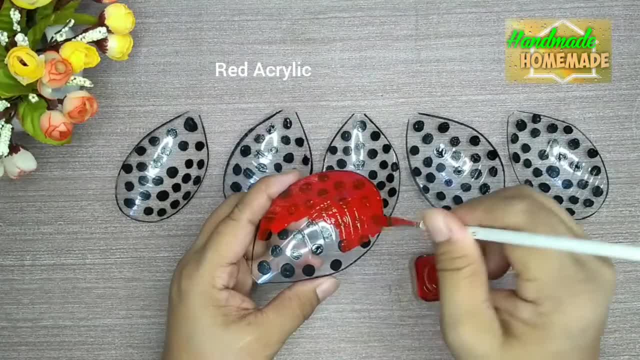 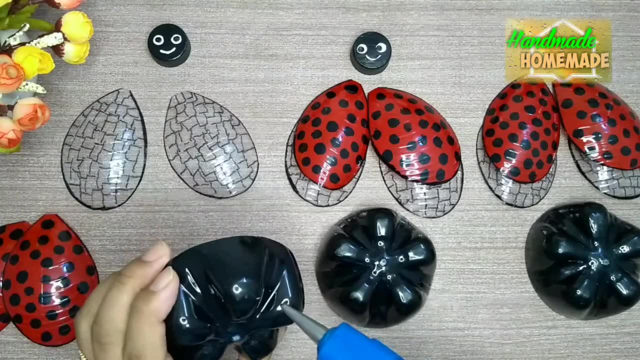 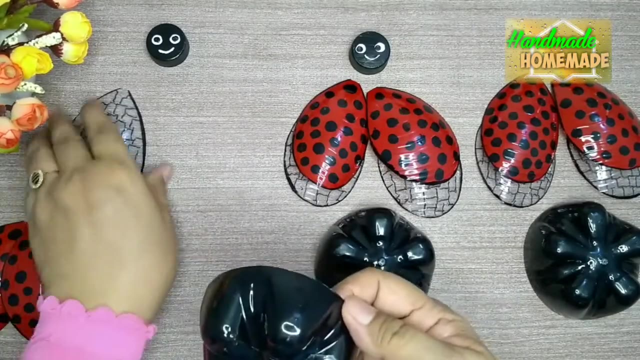 What do you do? what do you do when you're going through? going through? I'm gon' dance like David. have faith like Abraham. Prophesy like Jeremiah: pray just like Elisha. I'm gon' dance like David. have faith like Abraham. 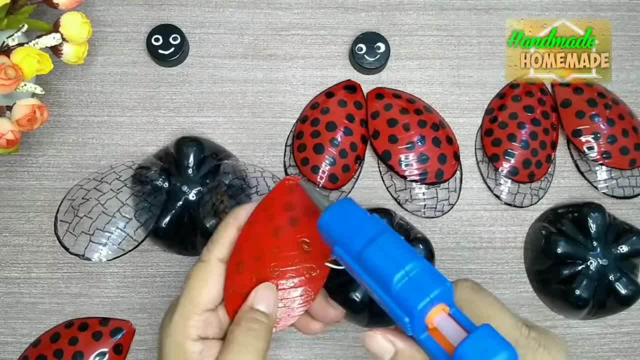 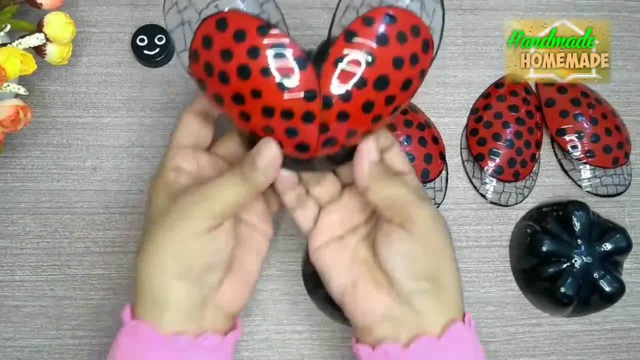 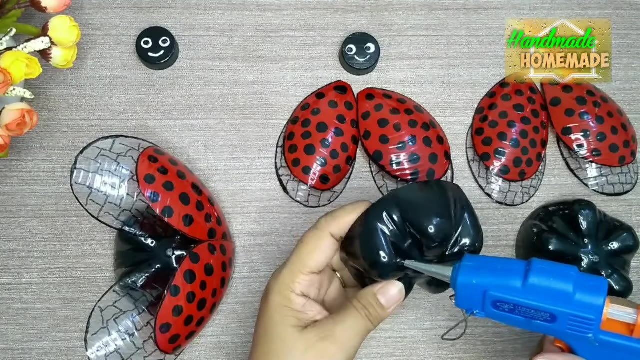 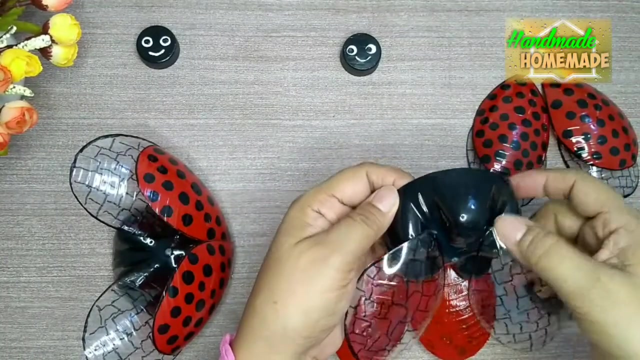 Prophesy like Jeremiah, pray just like Elisha. Mind don't for matter, it don't matter. So do you mind if I just give you all the praise I have inside? Never mind, never mind. Tell the things going on right now, I just wanna say hallelujah, hallelujah. 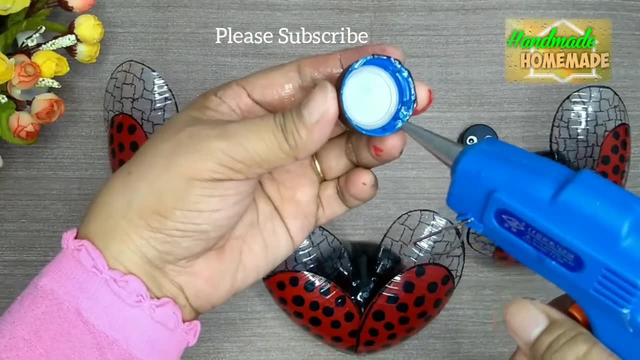 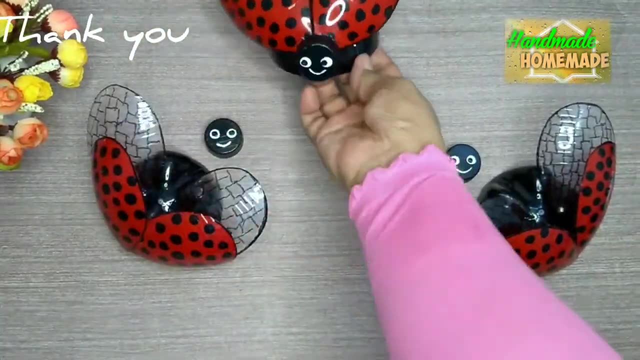 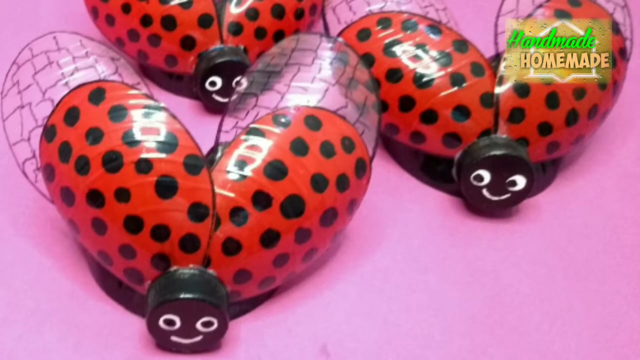 Praise the Lord, praise the Lord, praise the Lord. Oh, oh, oh, Cause what you're doing now. oh, oh, oh, I'm doing what you made us do. I just want to say hallelujah, hallelujah.